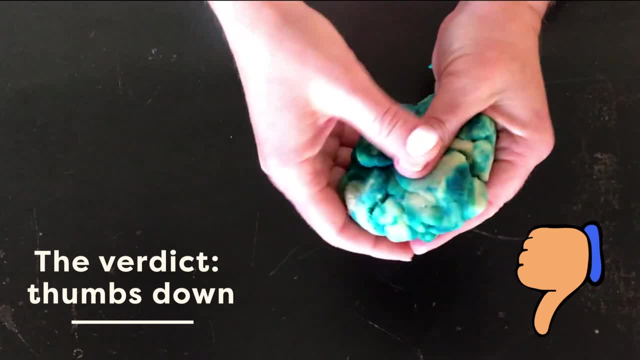 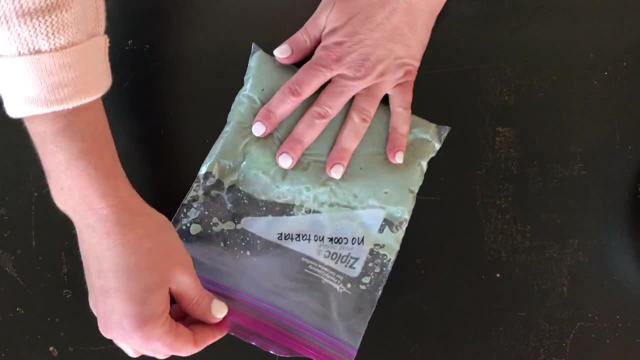 It really just doesn't seem like everything came together. This recipe was also no-cook and it also didn't use cream of tartar. You can see that it's just kind of squishy and oily. I don't even want to get it out of the bag because it's such a mess. 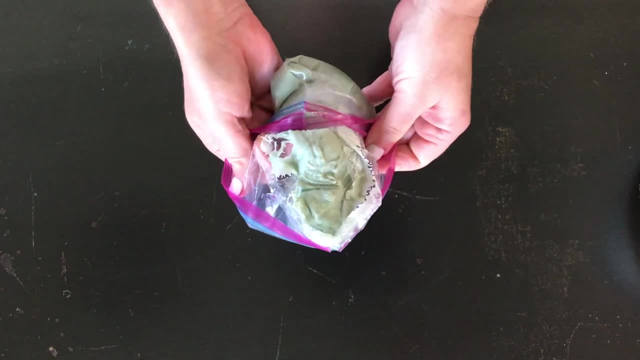 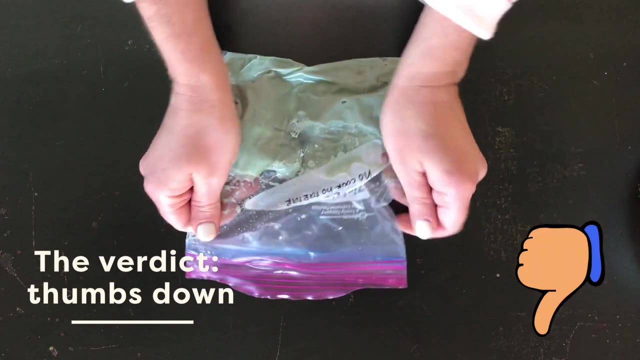 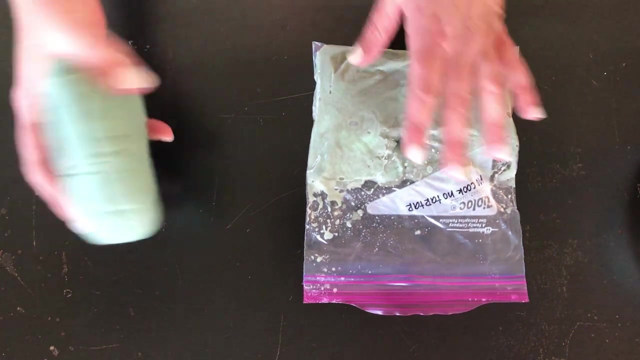 So again, maybe you would call this slime. I just think it's kind of messy but it's definitely not Play-Doh. Now, if you will look at that and compare that to the recipe I used from my mom's- her original Play-Doh recipe, 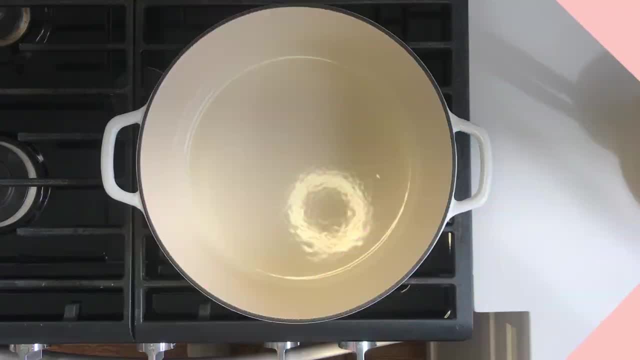 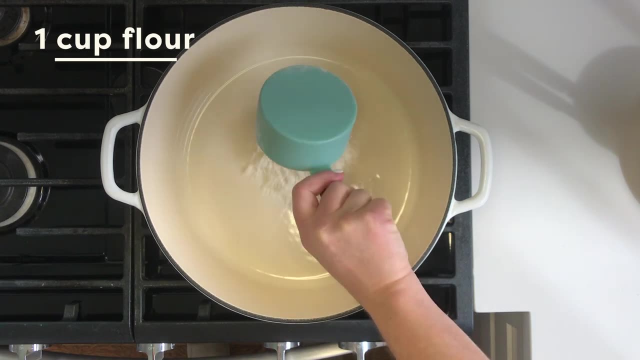 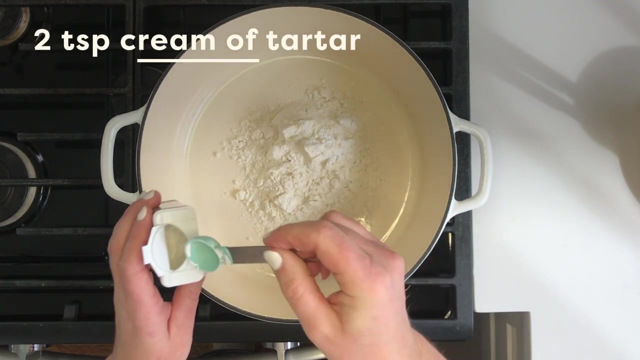 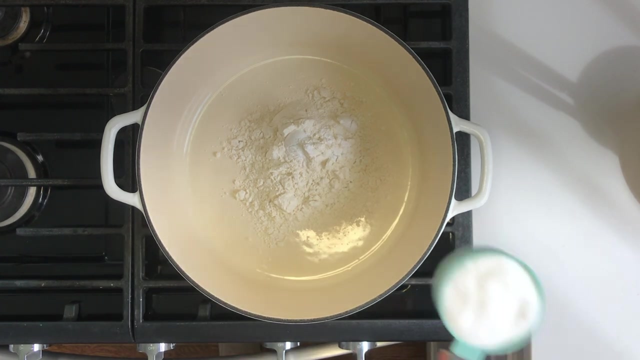 and you can definitely see the difference. Okay, step one is to use a heavy bottom pan, and we're going to add one cup of flour, two teaspoons of cream of tartar- and this can just be found in your baking aisle- and a half cup of salt. 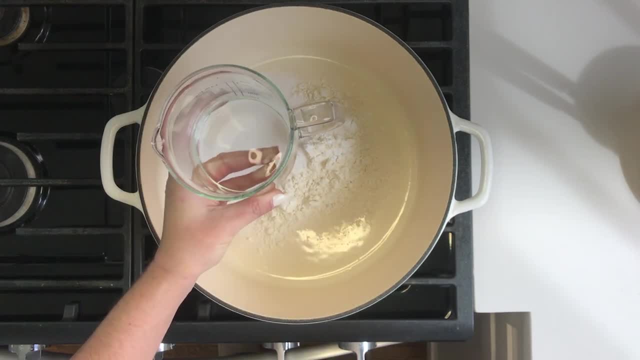 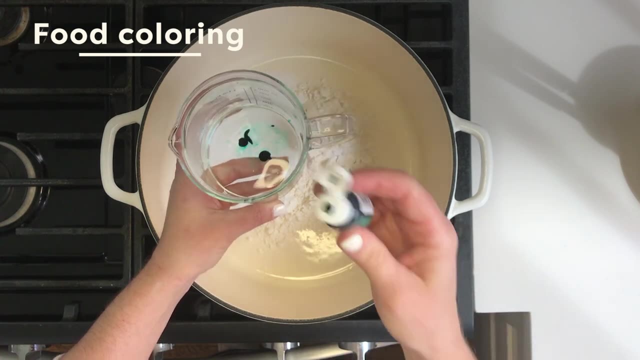 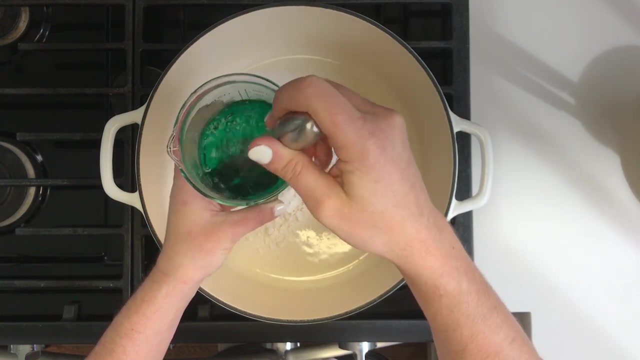 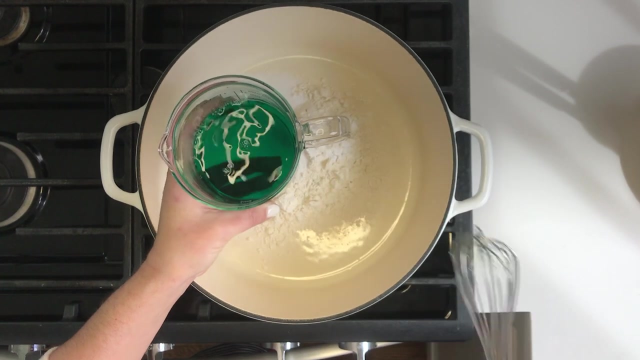 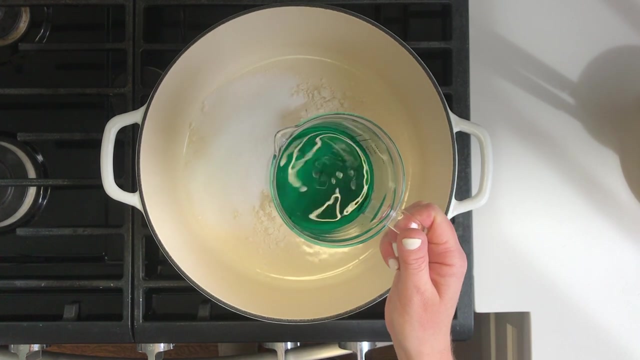 Next we're going to add our water. one cup of water And a pro tip here. add your food coloring, just a couple drops to your water and mix it in. now Let's give the 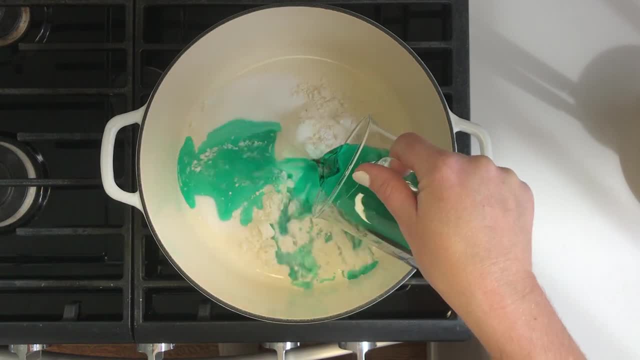 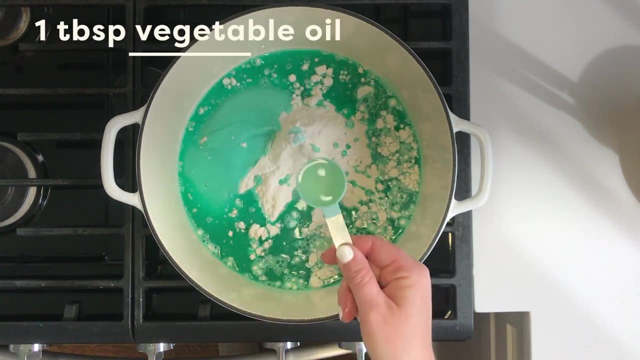 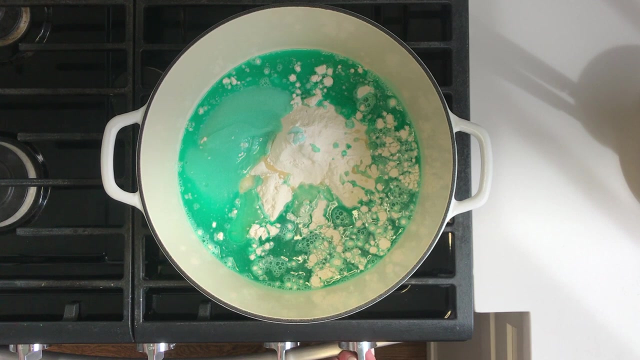 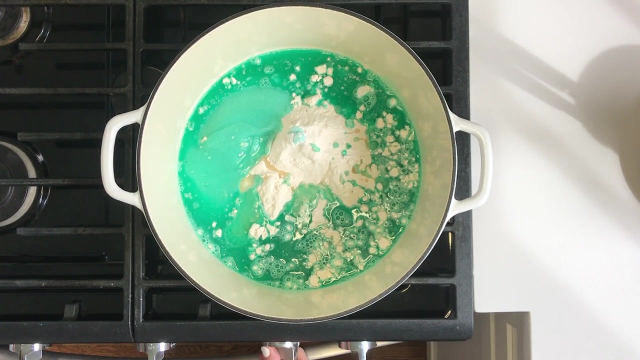 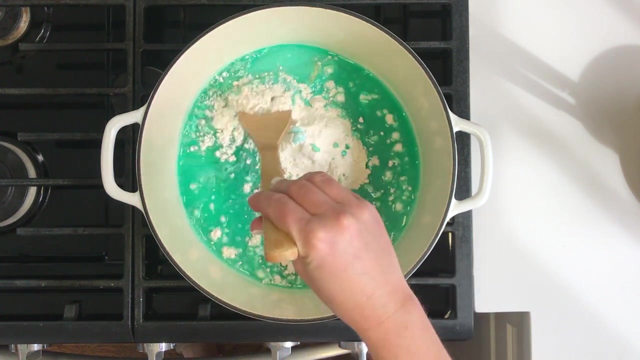 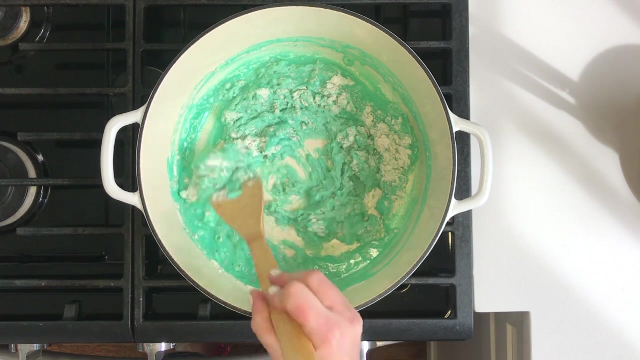 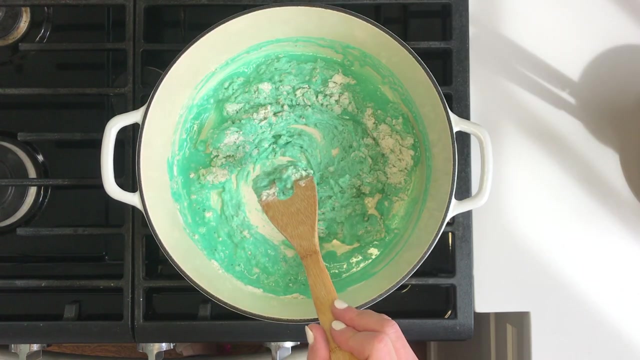 We're going to keep stirring this until it starts to become a solid, and you can see that it's getting thicker. We're going to keep stirring this until it starts to become a solid, and you can see it's. 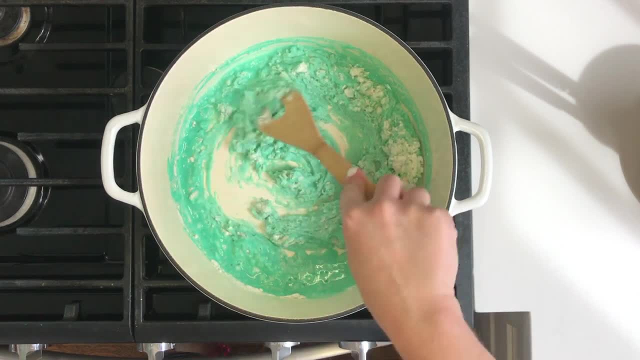 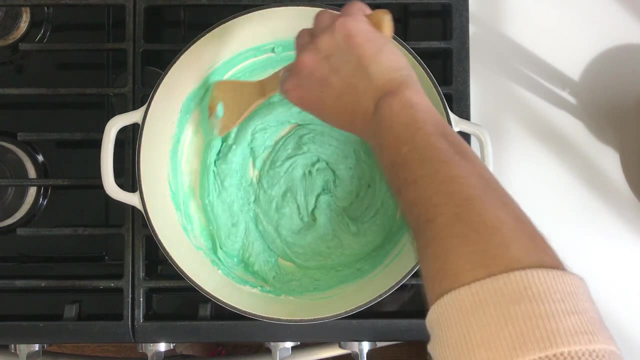 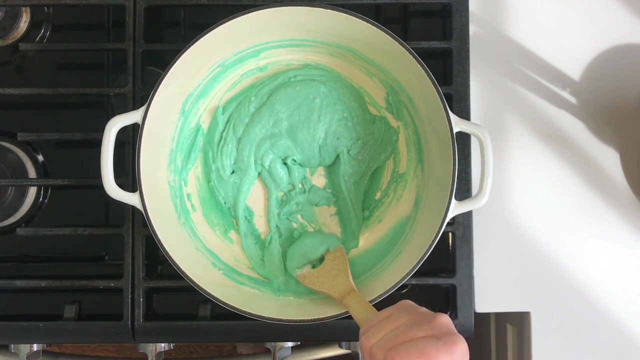 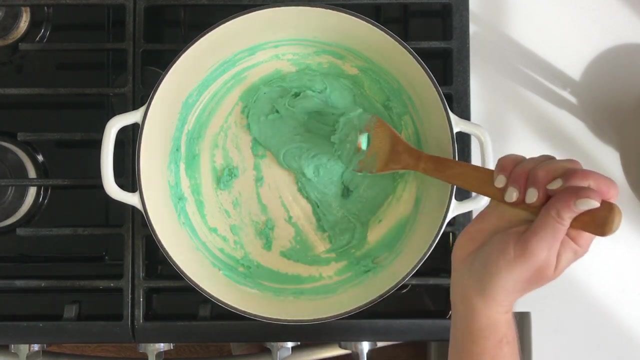 getting thicker and lumpy. This is how it's supposed to look. Just the smell of this brings back so many childhood memories. We did this all the time. Okay, it's starting to come together. See how it's starting to kind of stick together and pull off the bottom. 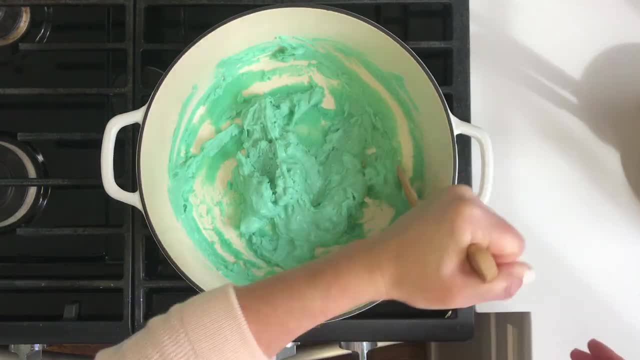 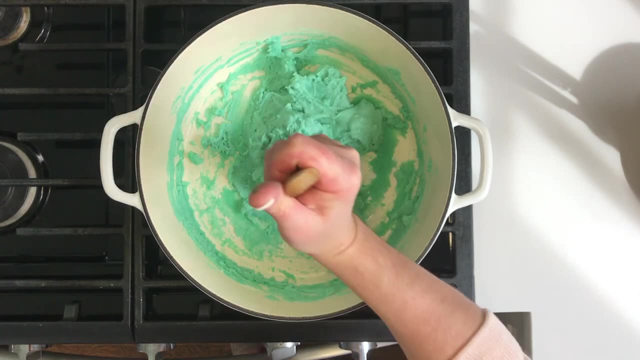 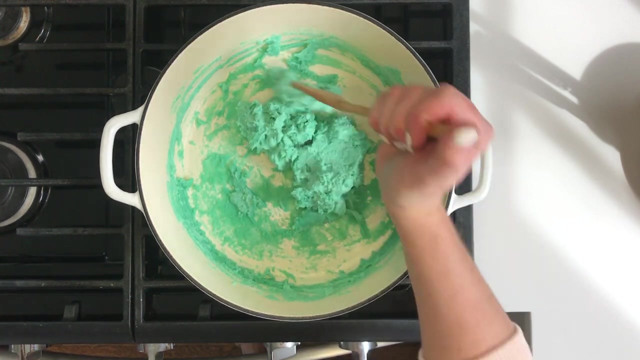 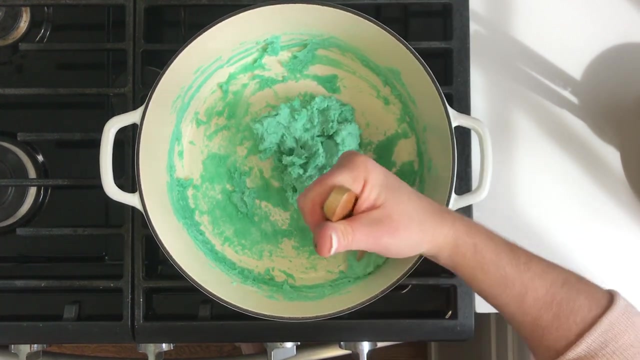 That's how you know it's getting close to done That right there is almost perfect. You know we are getting close to being done. See how it all just sticks together and makes one little mound of dough. I'm going to scrape what's off the sides. 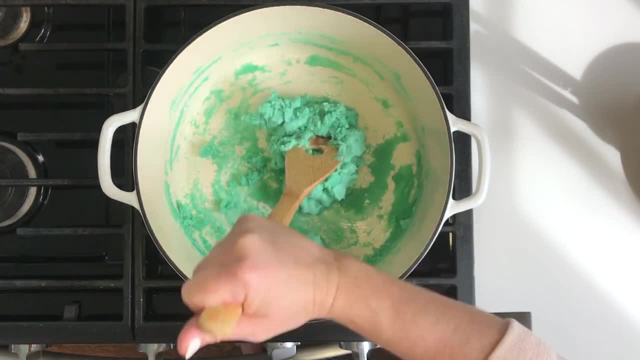 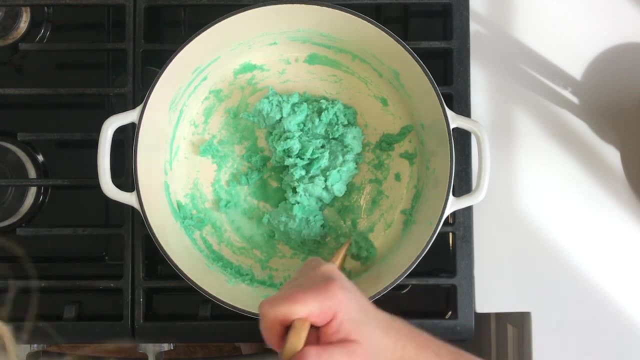 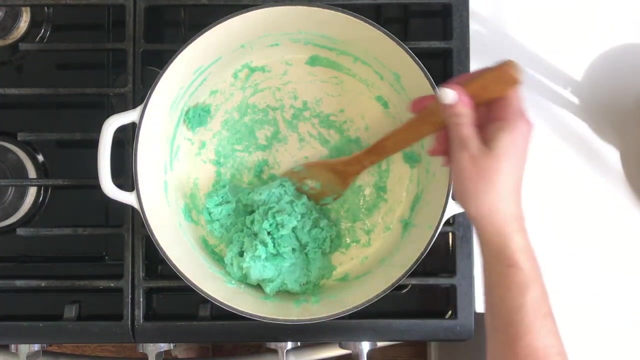 You see that It just starts forming together. I'm going to turn our burner off. get as much together as we can. This is hot, so be careful, and this is definitely a job for an adult to do. See that nice big mound of dough. 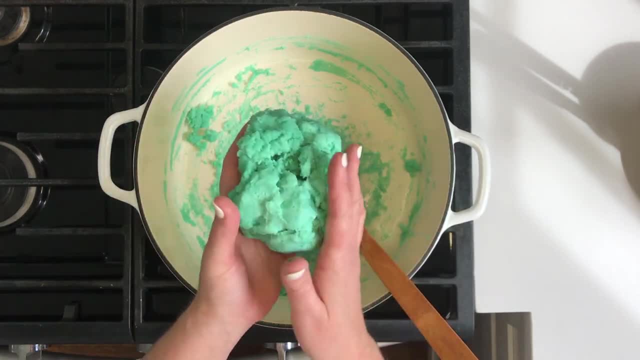 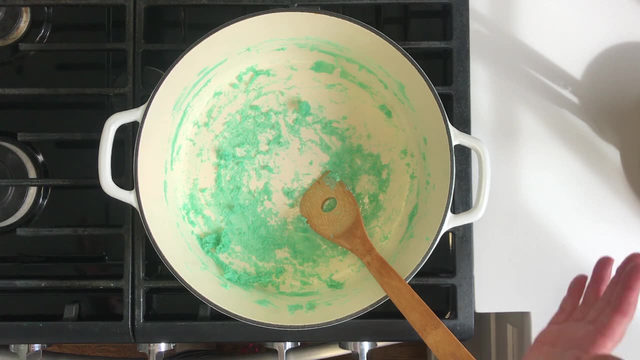 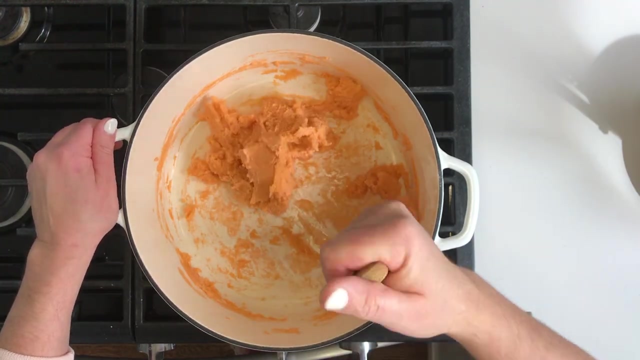 Now we're just going to set this aside on a plate or a piece of parchment or wax paper and we're going to let this cool completely Start to finish. I think that took under five minutes. so I'm going to go ahead and wash out this pan and I'm going to make a different color. 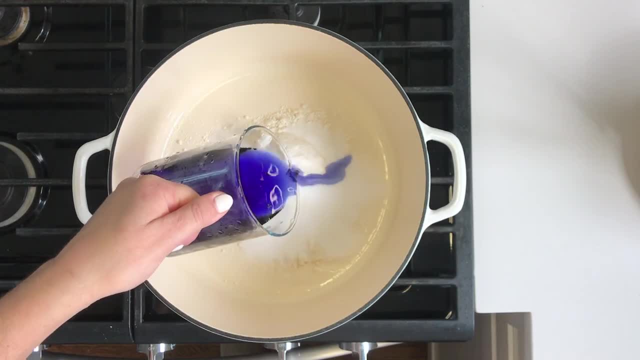 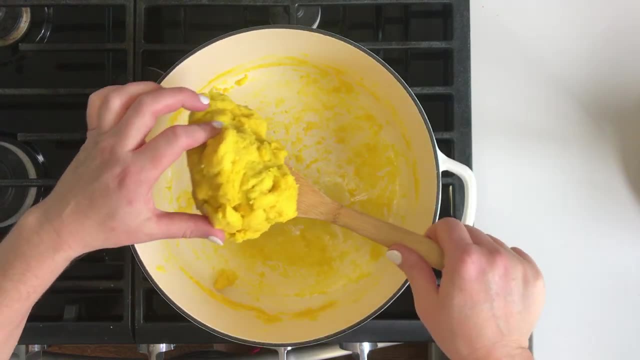 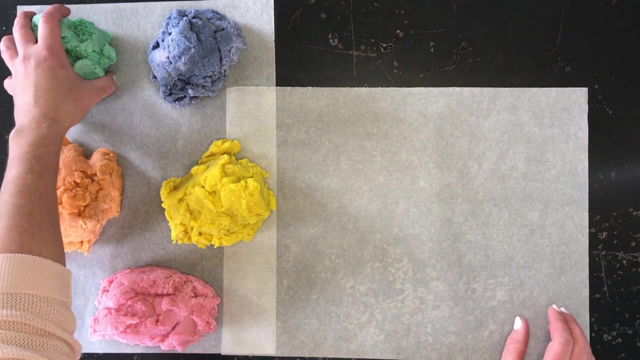 Alright. so I've made all my colors and they've been sitting to cool. Now all I'm going to do is knead them to mix them, And this is a fantastic job. for little waffles- I love it. Little hands, They love it. 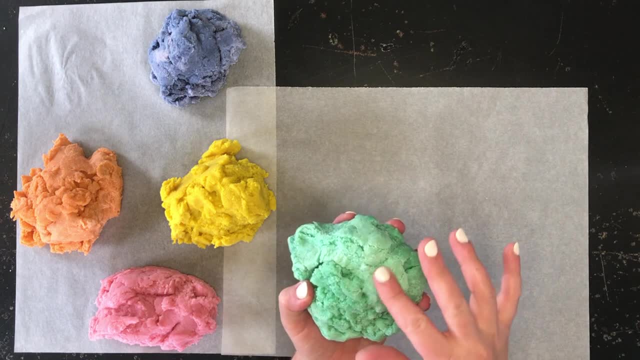 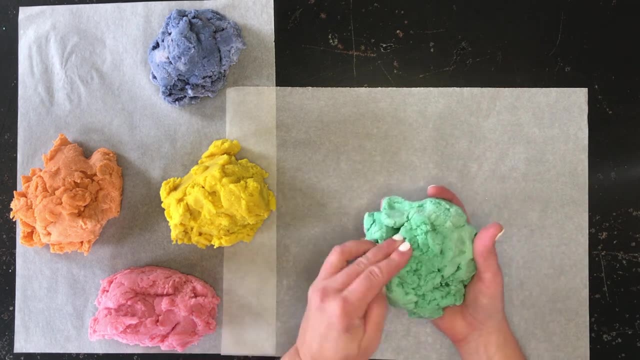 So I'm hoping you can see, now that they've been sitting for a while, they kind of got a little bit of almost like a salty crust on them. but so that's why it's important to knead and really mix all this stuff around before we start playing with it. 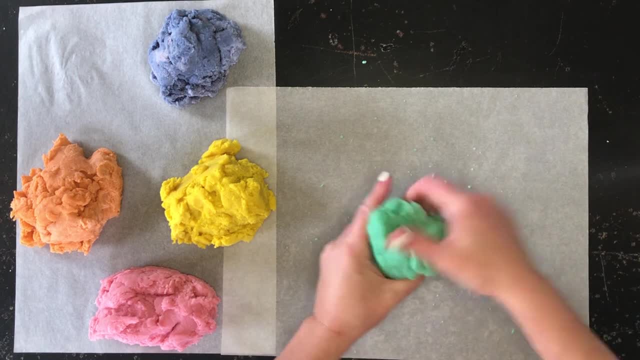 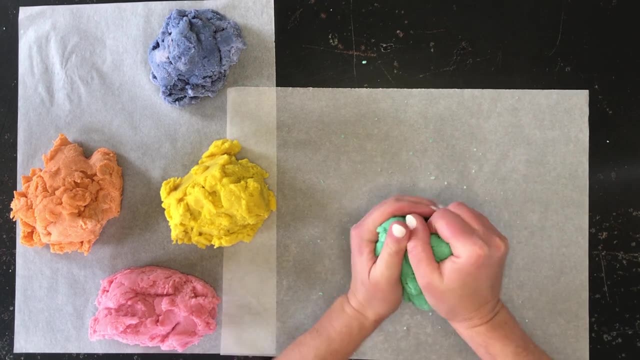 Now, if you put this in an airtight container like a plastic bag or a container with a lid, this stuff will keep for months and months and months, And look how much more you get than one of those containers you buy from the flea market.